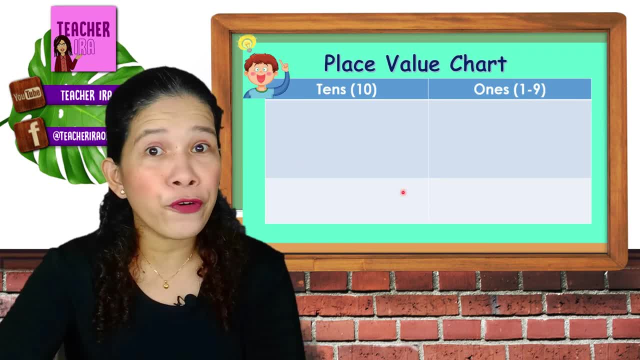 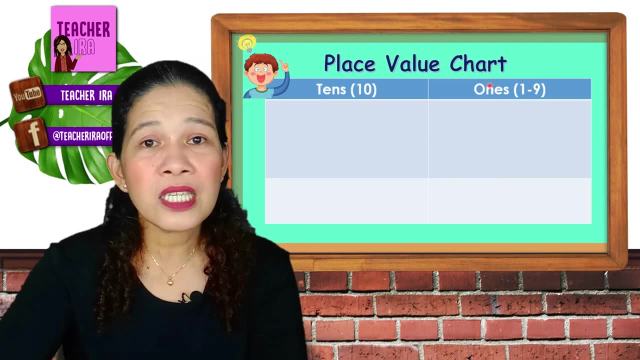 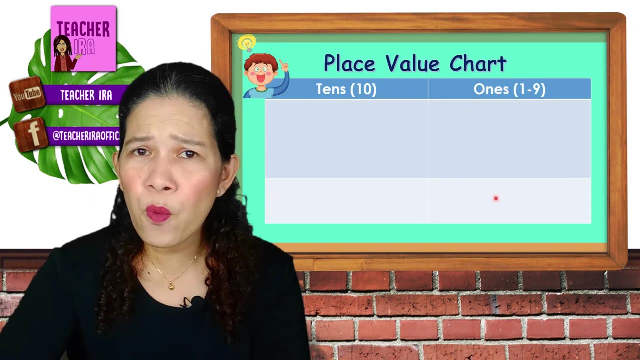 As you can see here, kids, we have two columns here for now because you are still in preschool, but when you go into further study there are more places after this. Okay, this place is called the ones place and this one is called the tens place. When you say ones, children, all the numbers that would be here are all with the value of itself. 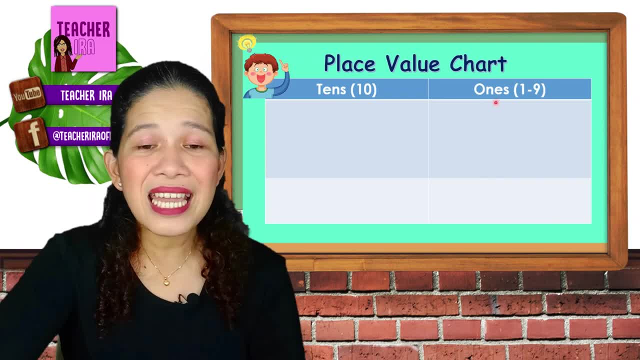 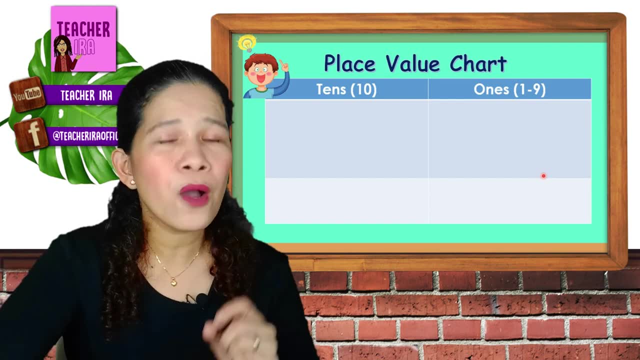 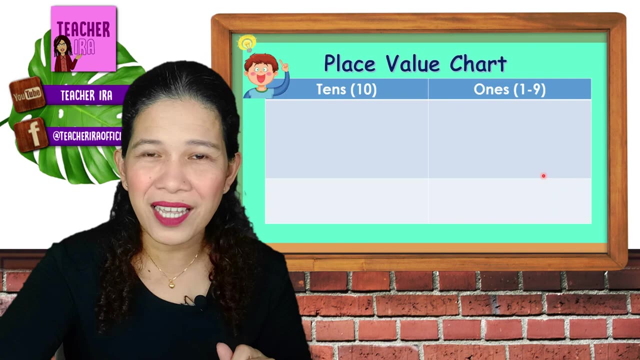 There is a rule that goes with it. Remember that each column or each column Place here would just have one digit. How many One digit? When you say one digit or digit means number. You cannot have two numbers in one place, So let's take a look at this one. I am going to use blocks to teach you this place value chart. 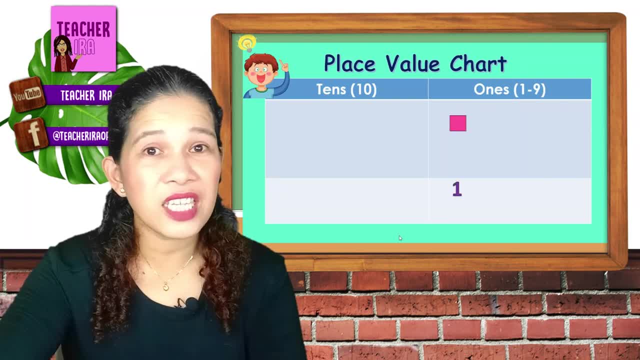 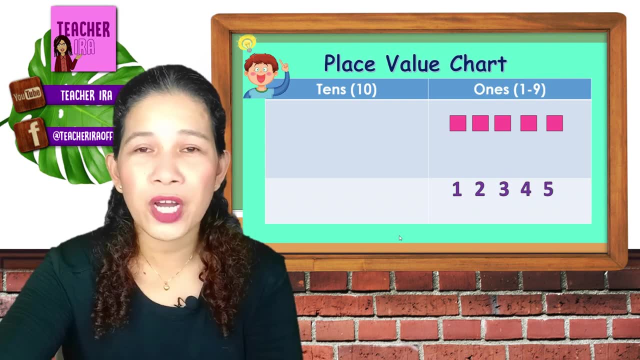 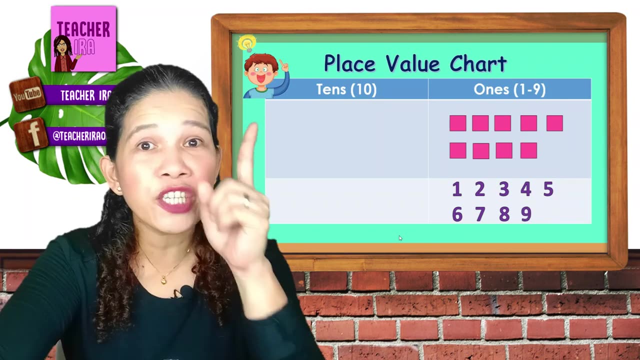 One- Okay, that could be there also, because that's in the ones place. It's the one, two, three, four, five- You come with me- Six, Seven, eight and nine, Remember, all these numbers are just with single digit or one number only. 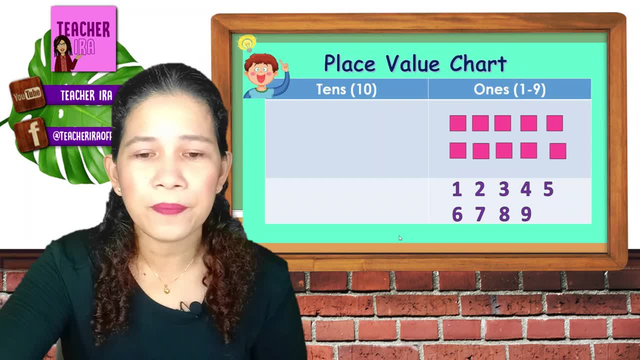 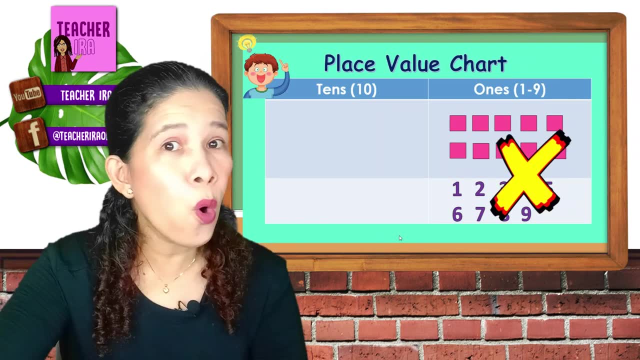 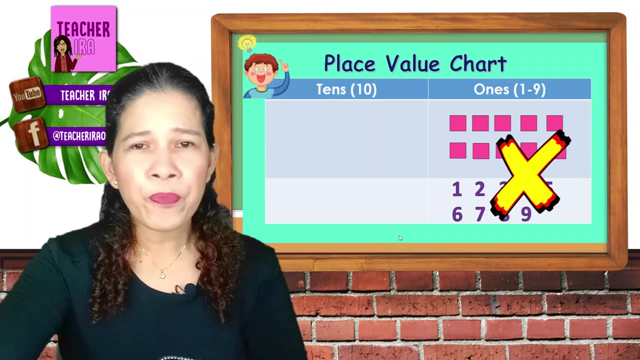 What if I would add another block here? whoa, that becomes ten. now Do you think I can write the number ten here? No, no, no, Because number ten has two digits already. So kids remember, when that becomes ten, that will be me. 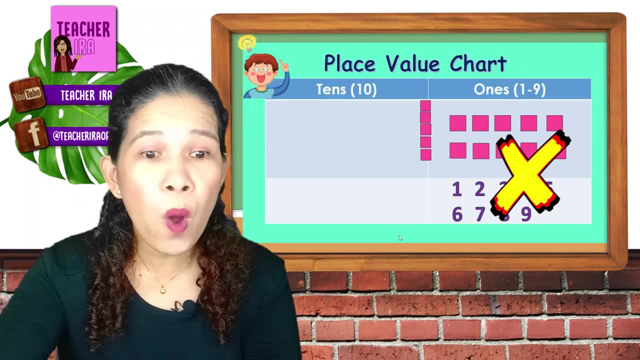 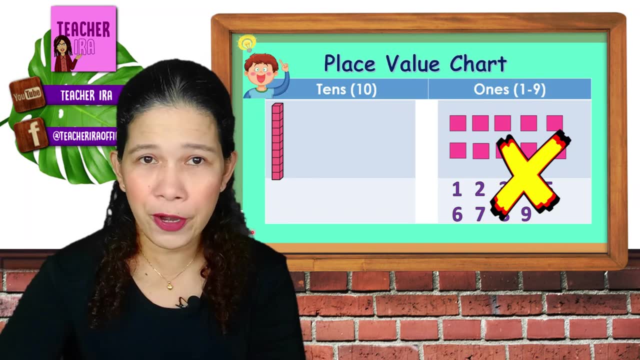 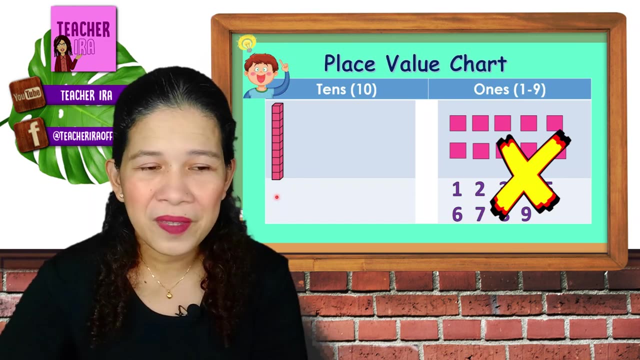 Remember when that becomes ten- that will be me. Remember when that becomes ten- that will be me- will pile up into one line like this: it will become a one stack and will be transferred to the tenth place. see now, here we have one stack of block and this is called 10.. okay, this is 110 now. 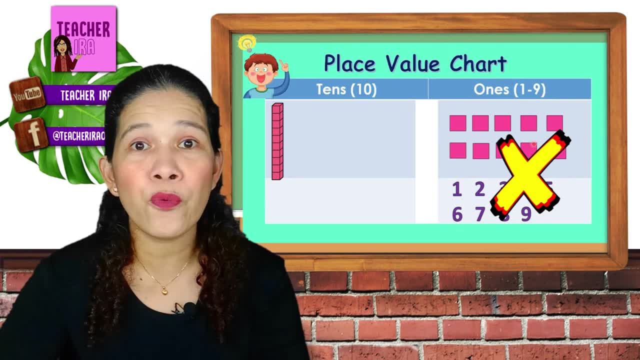 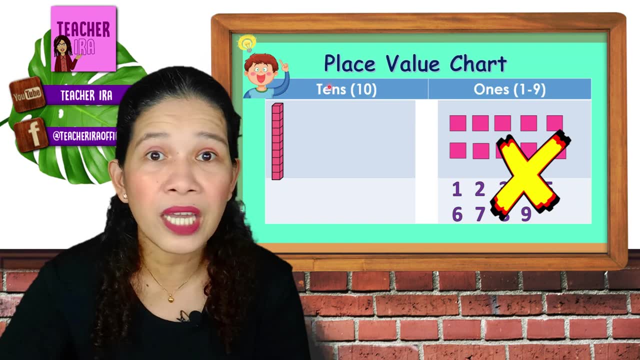 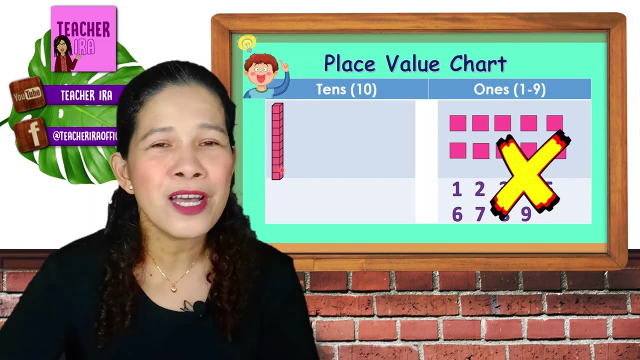 meaning all the numbers in the ones place are with one, one, one, one one. you will count it as it is, but the numbers in the tenths place will be counted by tens. okay, the value now or the meaning of the numbers here would be by ten. okay, so when you see one here, that means one, ten. when you see two, that. 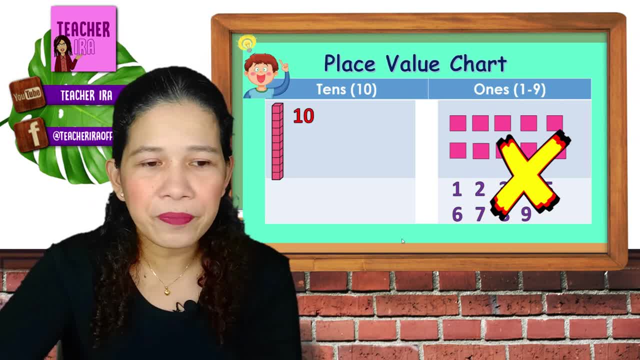 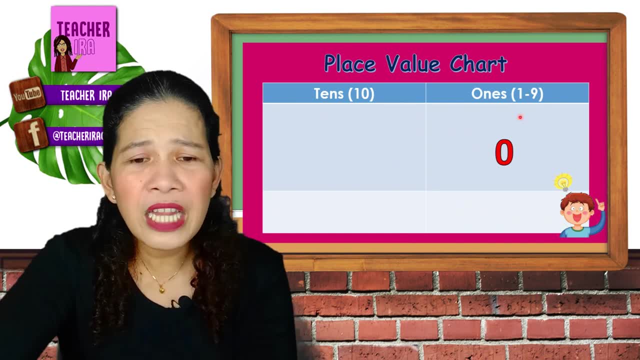 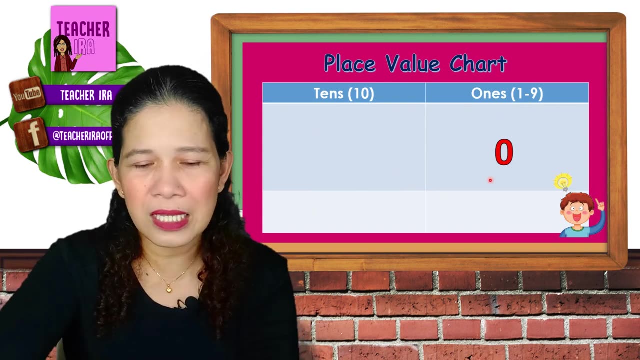 means two tens. let us try. okay, let me show some more. okay, that means one ten, and one ten equals ten. now I will have your zero in the ones place, but we will just move on to the tenths place because the ones place is just easy. okay, so here i will have one, two, two stacks of blocks here, meaning that's ten, twenty, ten plus. 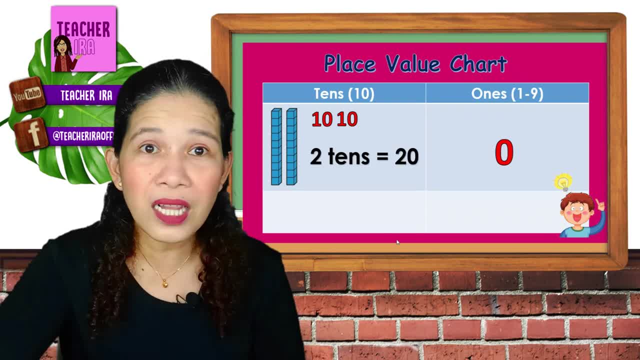 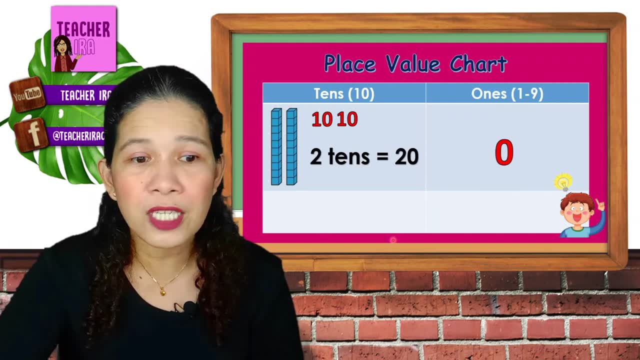 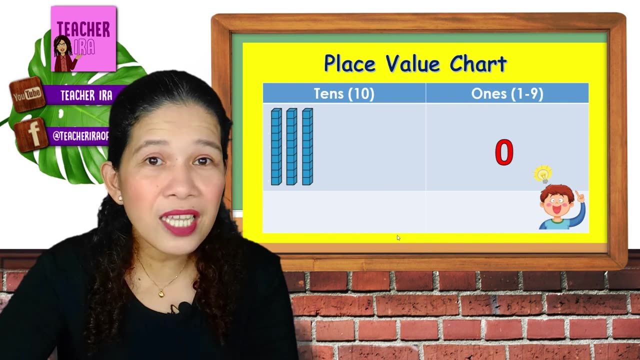 ten, and then we'll have two tens equals twenty, so you will call it now twenty. since we have zero in the ones place, this will just be called twenty. now let's add some more: one, two, three, three stacks now. now let's have one or ten, twenty, thirty. how many tens are there? very good, so there are three tens. 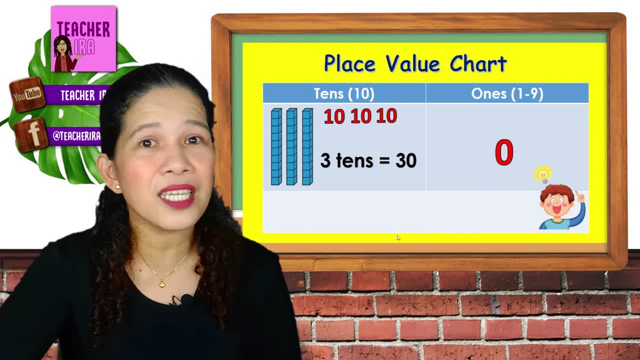 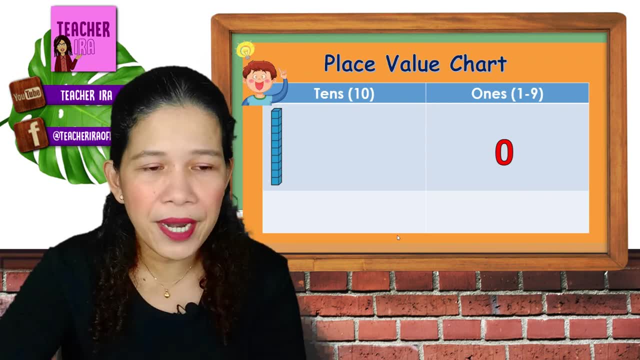 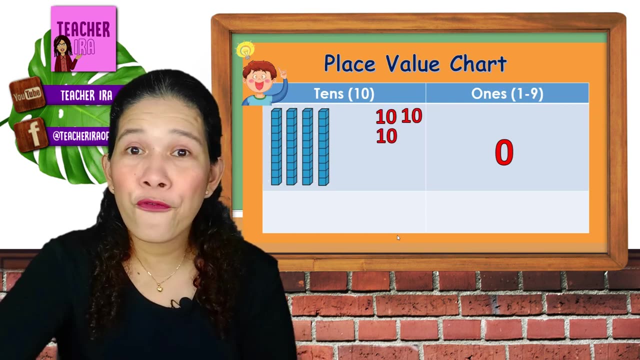 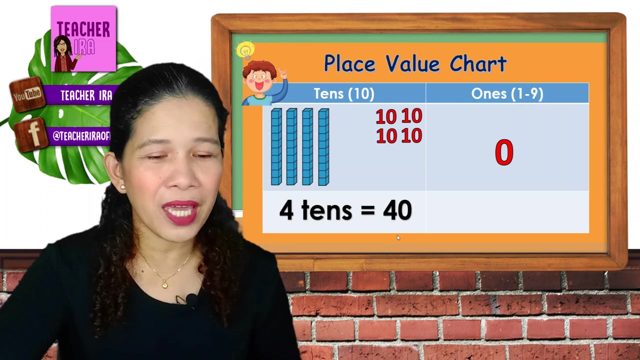 meaning that is thirty. three tens equals thirty. okay, now let's have this one. let's count the tens now: one, two, three, four. now let's give the value 10, 20, 30, 40.. okay, that's four tens equals 40.. very good, is it getting clearer now, kids? now let's have some more blocks here. 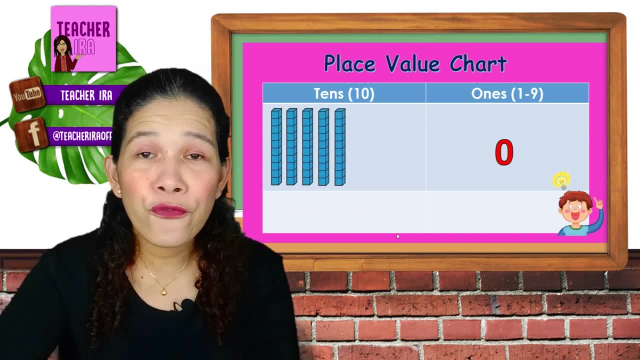 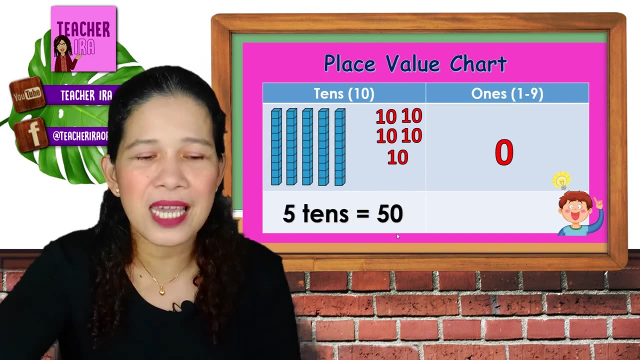 one, two, three, four, five stacks of blocks. let's give the value 10, 20, 30, 40, 50. so when you see five stacks of blocks there, that means that's 50.. five tens equals 50.. okay, now let's move on. 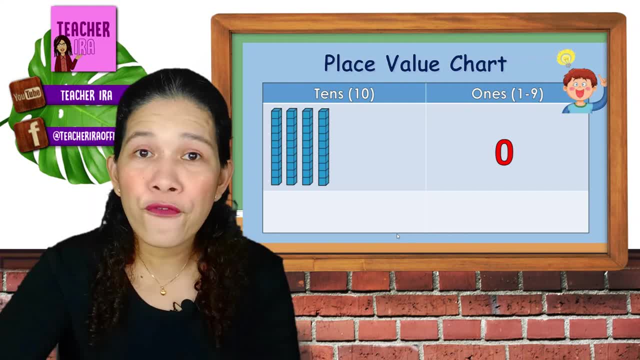 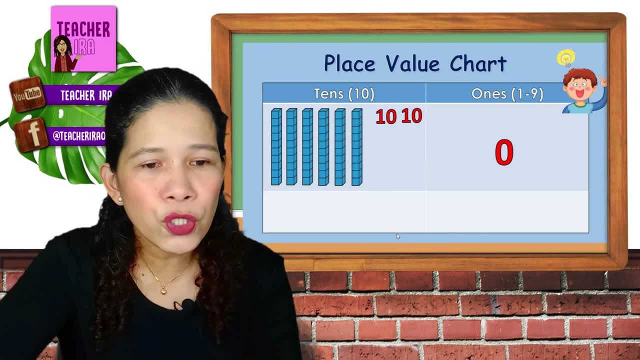 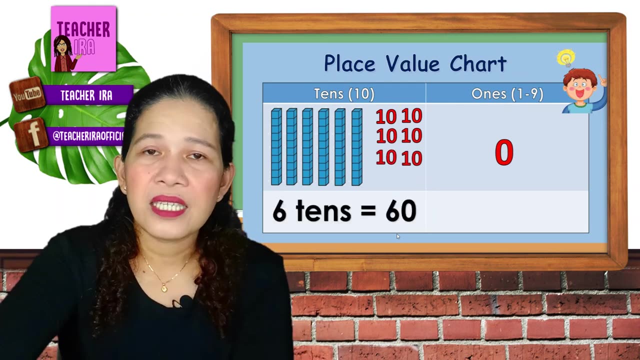 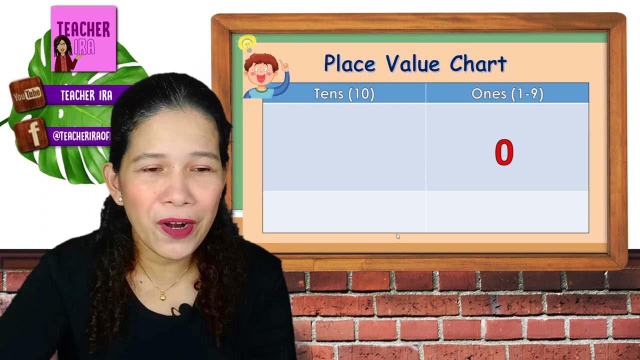 one, two, three, four, five, six. there are six stacks of blocks. now let's give the value 10, 20.. how many tens? yes, six, thirty, forty, fifty, sixty, six tens equals sixty. that's 10, 20, 30, 40, 50, 60. very good, let's add some more: one, two, three, four, five, six, seven. how many? 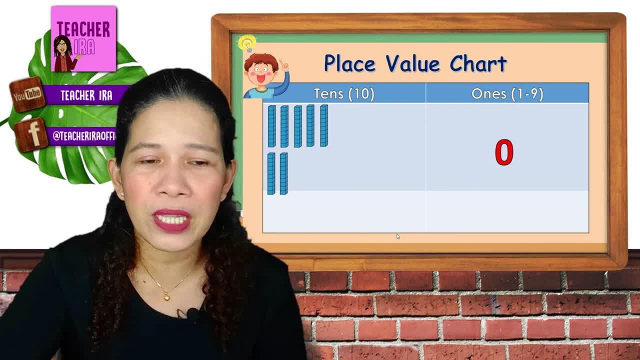 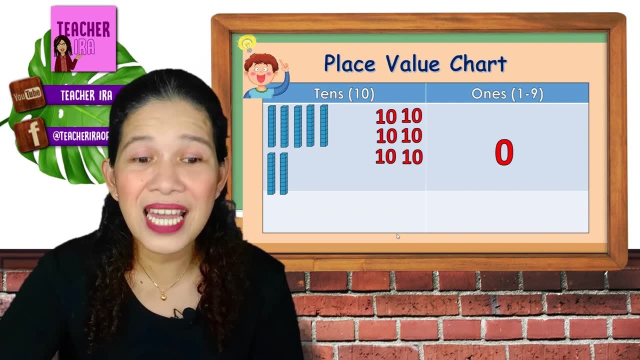 stacks of blocks. now, very good, seven. so let's give the value 10, 20, 30, 40, 50, 60, 70.. wow, because seven tens equals seventy. so easy. 10, 20, 30, 40, 50, 60.. wow, because seven tens equals seventy. so easy, that's. 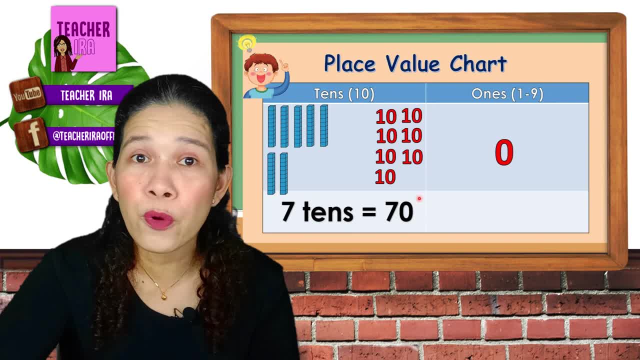 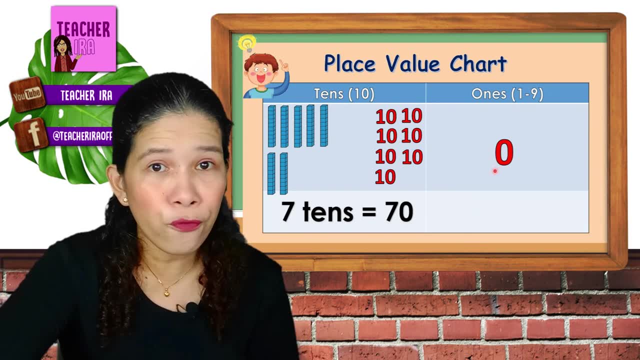 Meaning you have 7 in the 10th place and 0 in the 1st place, because we didn't write anything here. If I would write 1 there, then this becomes 1.. If I would write 4 here, then this becomes 4, because this means 1, 1, 1,, 1, 1 only. 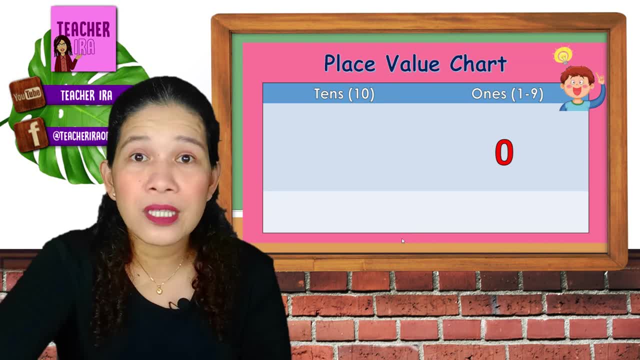 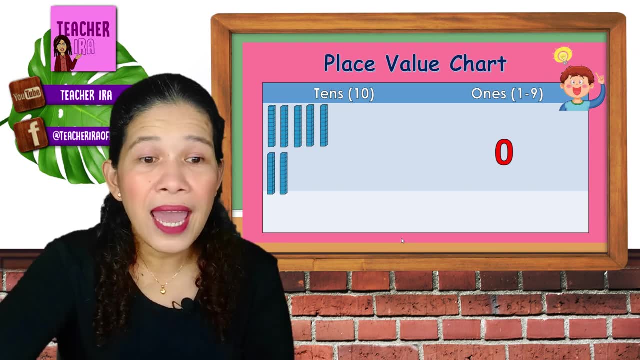 Let's move forward. Let's have some more stacks of blocks: 1,, 2,, 3,, 4,, 5,, 6,, 7, 8.. Wow, how many stacks of blocks are there? Very good, that's 8.. 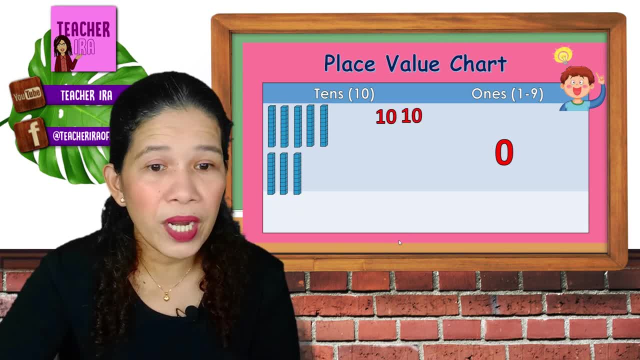 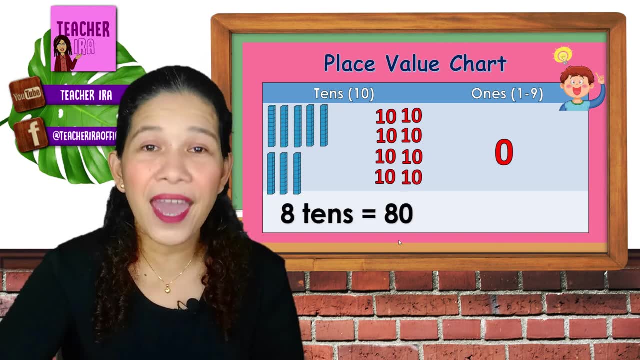 Let's give the value, So that's all: 10,, 20,, 30,, 40,, 50,, 60,, 70, and 80. Meaning, 8 tenths equals 80.. Wow, we're getting nearer. 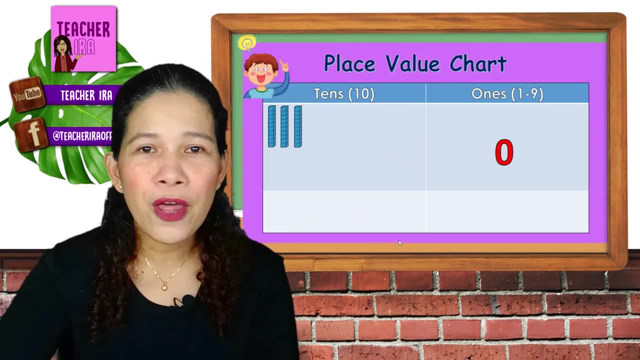 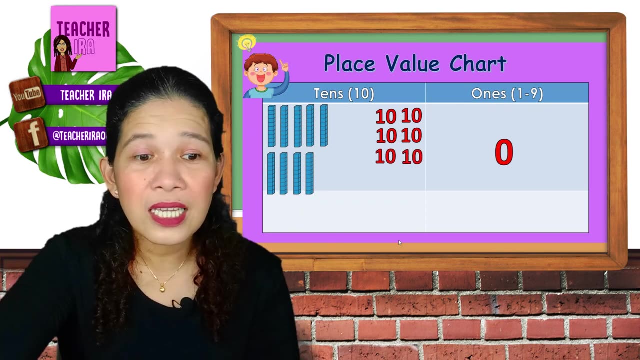 How about if I have 1,, 2,, 3,, 4,, 5,, 6,, 7,, 8.. 9,, 9 stacks of blocks, 10,, 20,, 30,, 40,, 50,, 60,, 70,, 80,, 90.. 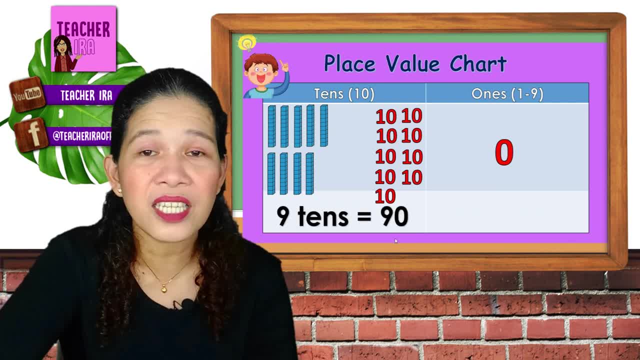 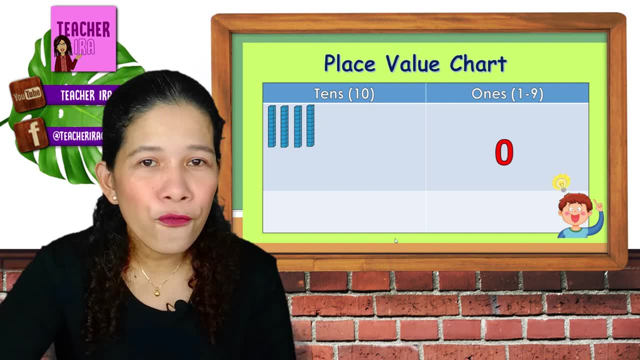 It's just 9.. So if we just have 9,, 9 tenths equals 90.. Next, 1,, 2,, 3,, 4,, 5,, 6,, 7,, 8,, 9, and 10.. 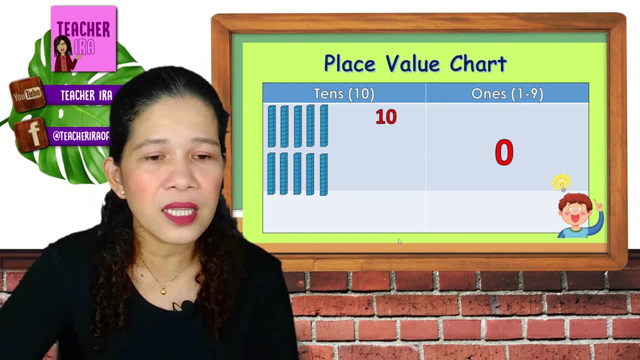 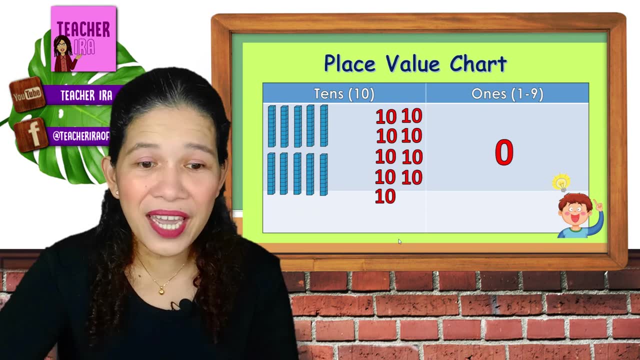 Oh, there are 10 tenths. Let's count them by tenths now: 10, 20,, 30, 40, 50,, 60,, 70,, 80, 90, 100.. Meaning, if you have 10 tenths, that means 100. 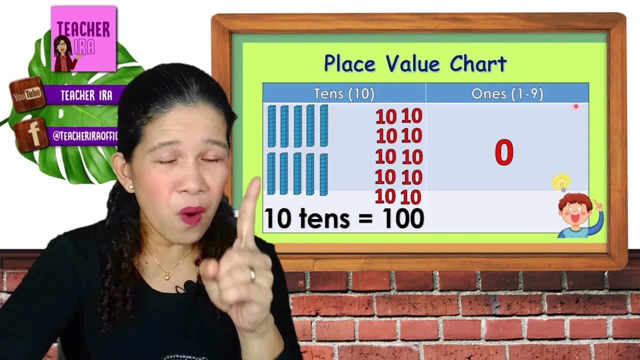 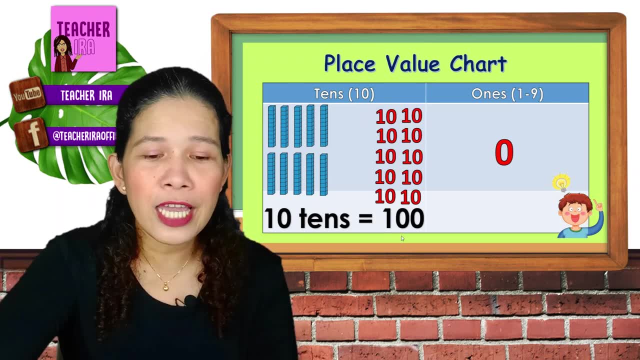 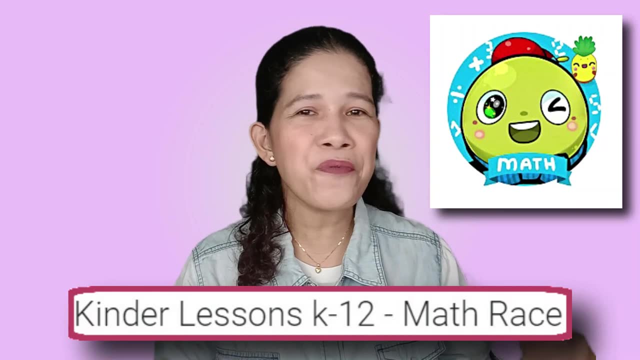 Wow, is it clear with you now kids, 1 means 1.. In tenths you would have all by tenths. Now let us try if you could answer this one. Hi, kids, This game is called KinderLessons- K-12 Math Race. 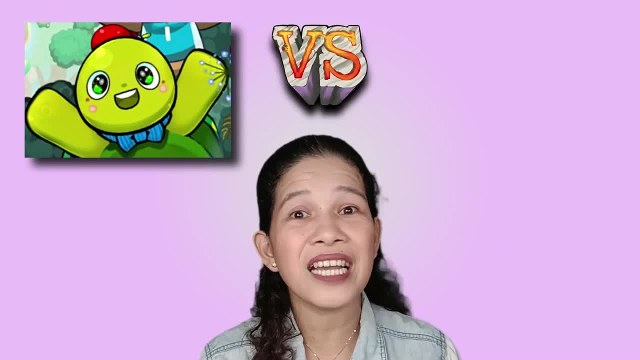 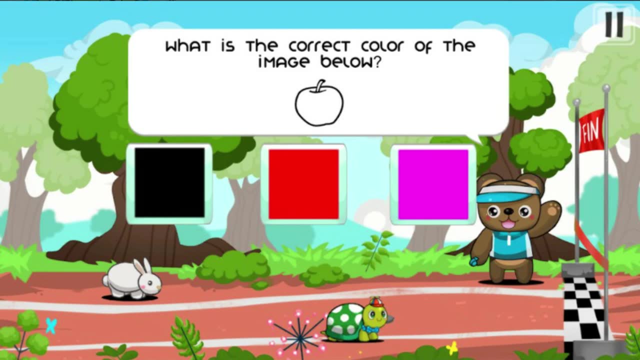 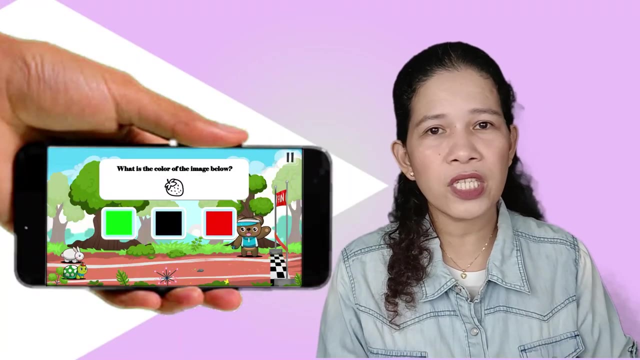 Here is Mr Turtle. Can you help him win the race against Mr Rabbit? Here's how to do it. Each race consists of different questions about math topics such as colors, numbers, shapes and many more. Mr Turtle takes a step closer to the finish line each time you tap the right answer. 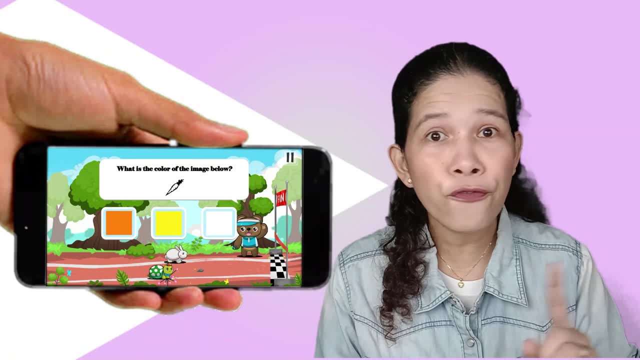 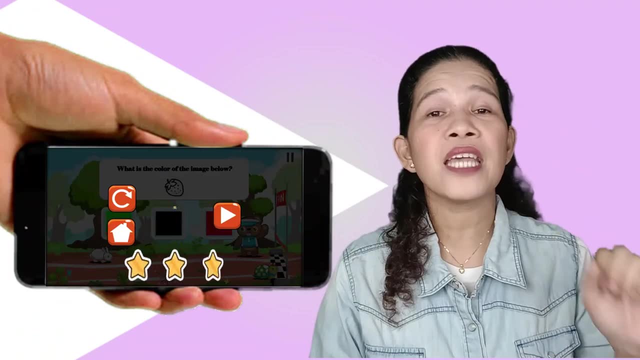 And Mr Rabbit would take a lead. If you would not be able to answer, you would be out. You would not be able to make the right answer. If you get the right answer, Mr Turtle would win with 3 stars and unlock the next stage. 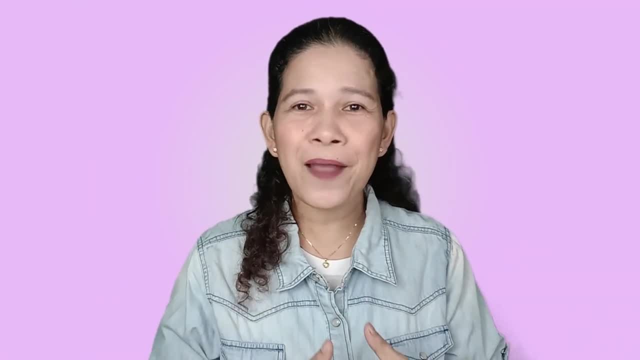 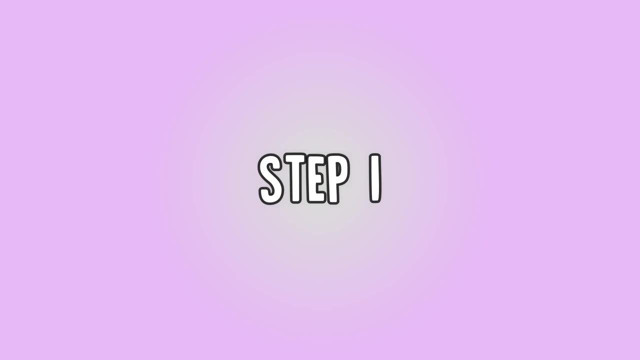 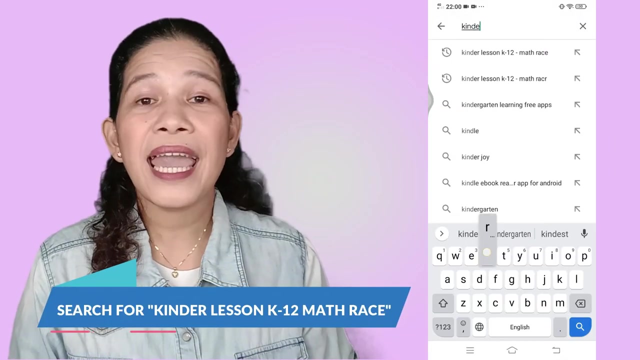 Kids. let us learn math while playing. And these are the steps that you should do to have this game: Number 1. Go to your Google Play Store- Number 2.- Tap the search box and type KinderLessons- K-12 Math Race. 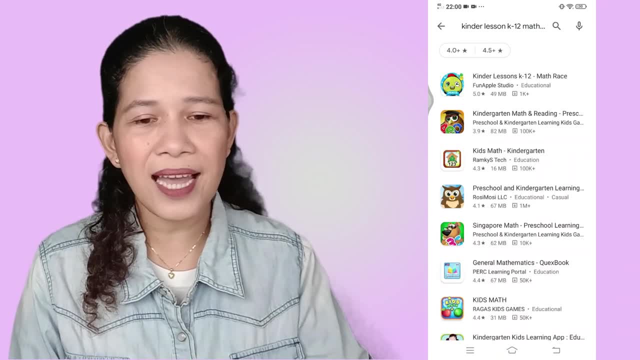 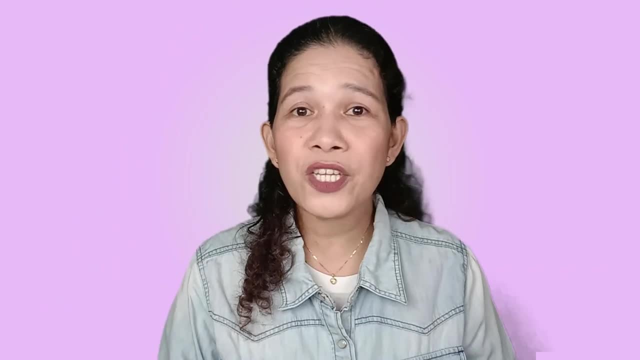 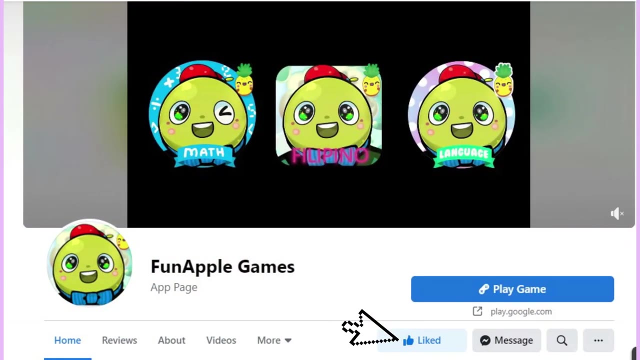 Then press enter or the small magnifying glass on your keyboard. Step 3. Click, install and enjoy. KinderLessons K-12 was made by PanApple Studio, So make sure that you visit their Facebook page for more game info. Here are the stacks of blocks. 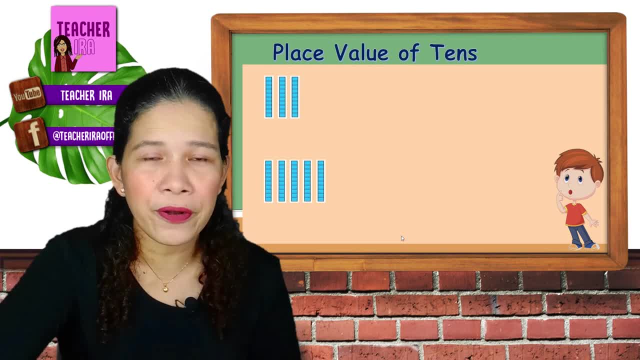 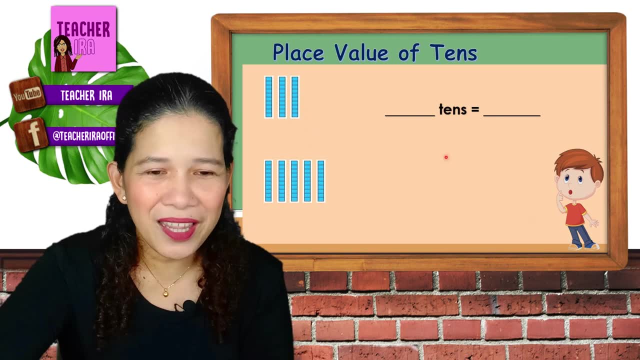 Let me see if you can find out how many tens are there. Let's count 1,, 2, 3.. You can do it by counting 1,, 2, 3.. How many? Okay, that's 3 tens. 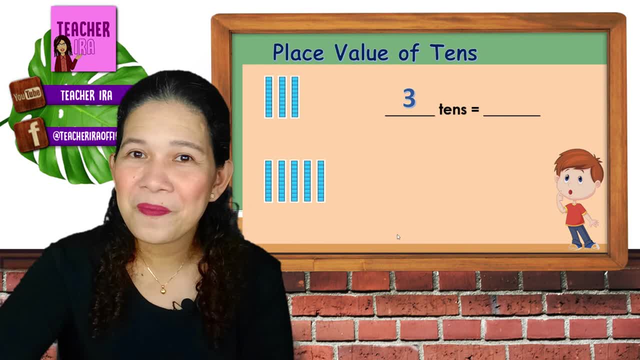 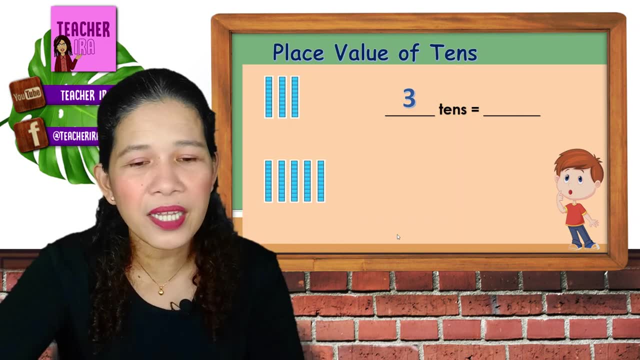 Meaning 3 tens equals Very good. So you're just going to write the 3 and then 0 because there are no 1s, So here is the 0. So we put here: 3 tens equals 30.. Great job. 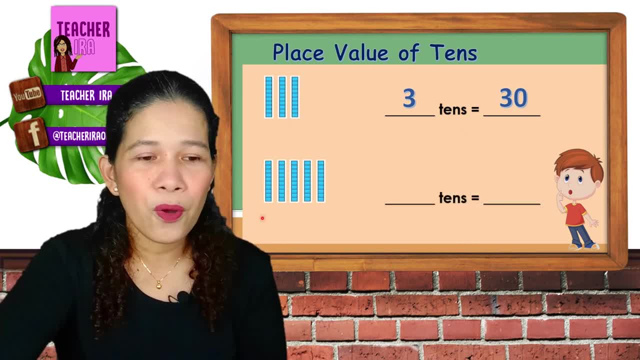 Now next one: How many stacks of blocks here Ready? 1,, 2,, 3,, 4, and 5. There are 5. And if you have 5 tens, what would be the number? Very good again, children. 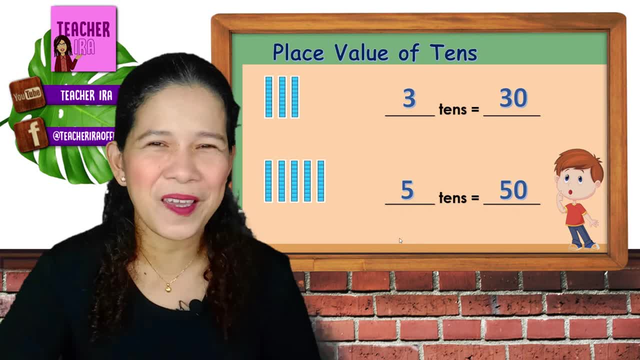 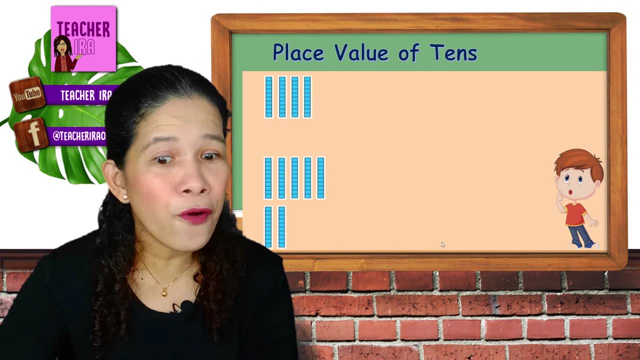 You got it right, That's 50.. Let's have some more, Yes, more examples. Okay, Let's count 1,, 2,, 3,, 4.. How many tens? 4.. And what could that be? 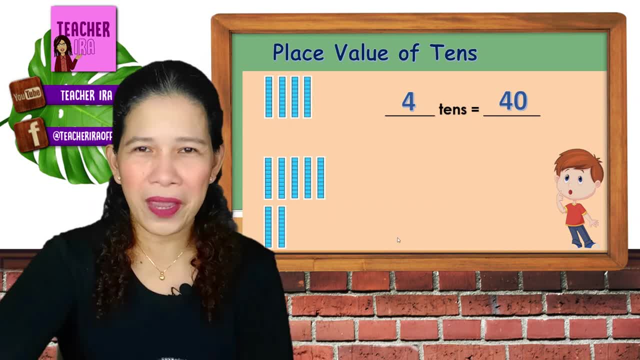 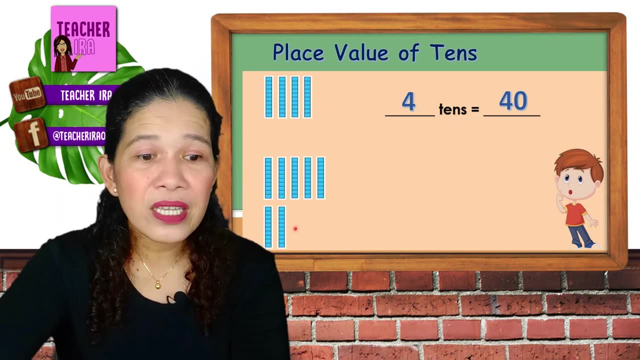 Very good, That's 40.. Very good, Great job. Now how about here? Let's count 1,, 2,, 3,, 4,, 5,, 6, 7.. Wow, 7 tens equals. 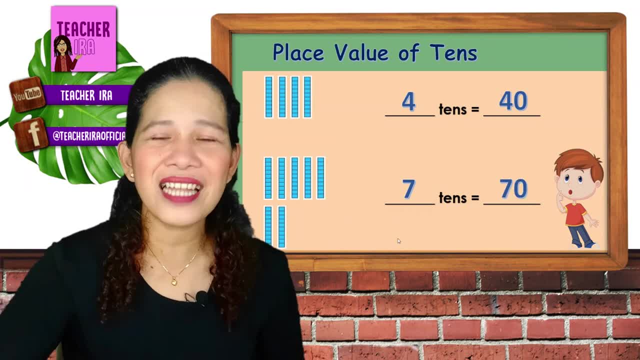 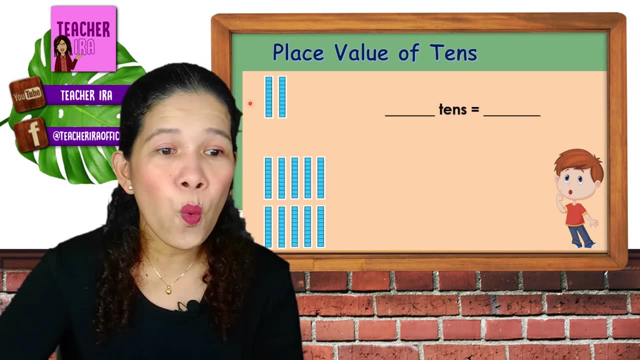 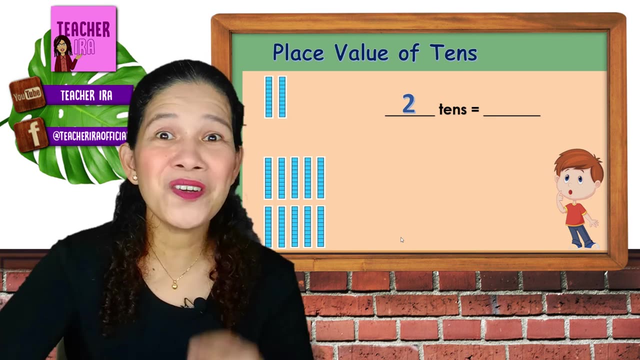 What's the number? You're correct, That's 70.. Next, how many tens are there? Let's count 1, 2.. So you got to write 2.. And what would be the number? You got it right. 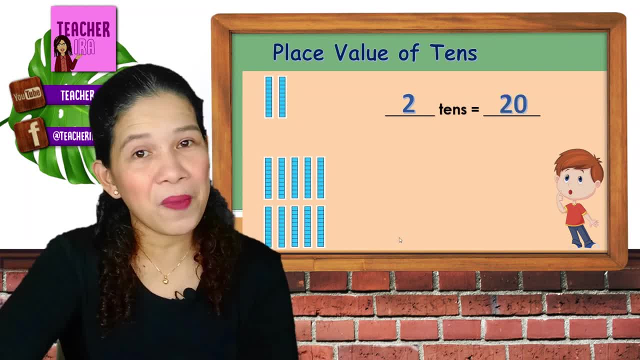 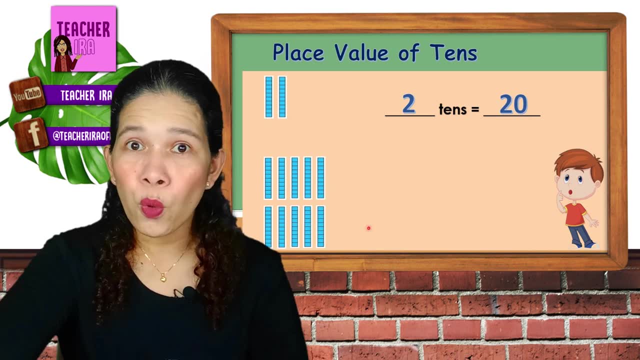 That's 20.. Yay, How about this one? 1, 2,, 3,, 4,, 5,, 6,, 7,, 8,, 9,, 10.. 10 tens, How many tens? 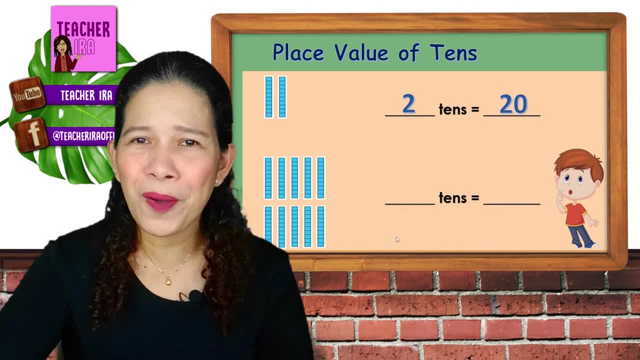 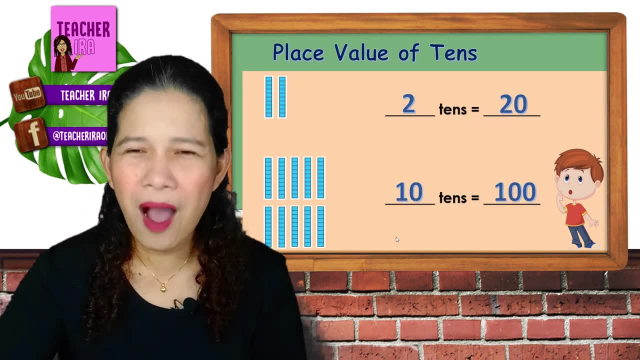 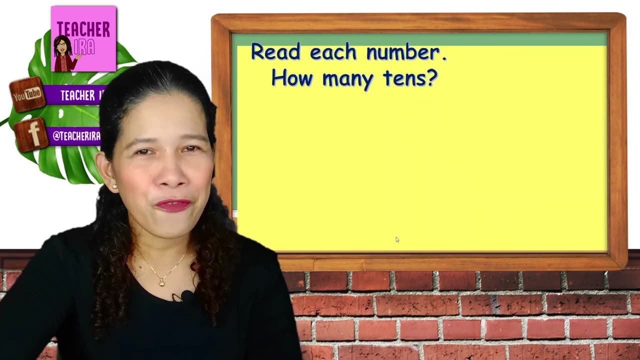 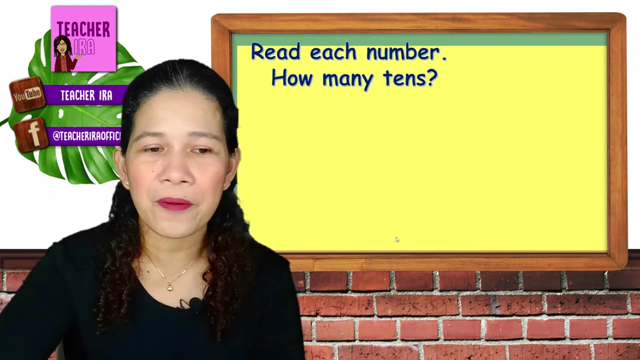 Yes, 10.. And what could be that number? You are absolutely correct: 10 tens equals 100.. Yay, Now let me see. Let me see if you really had understood the lesson. Read each number and tell me how many tens are there. 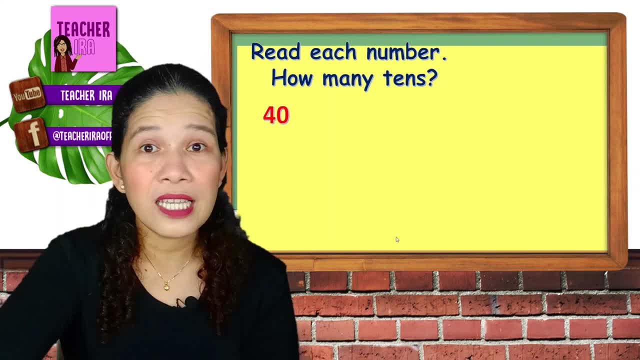 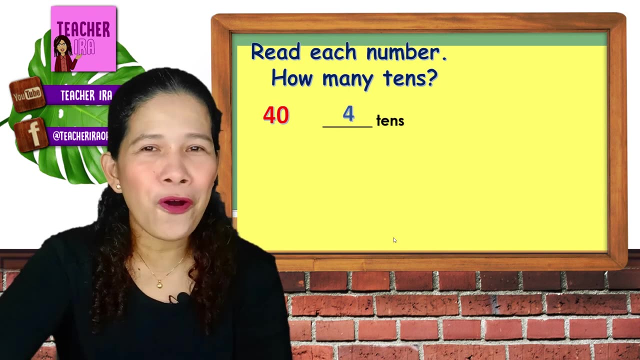 What is that number? What is that number? Can you read Correct? That's 40.. When you have 40, how many tens are there? Yes, That's 4.. You got 4 tens. That's why you had 40 minutes. 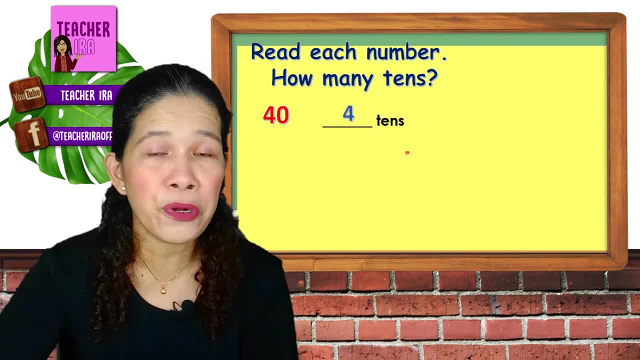 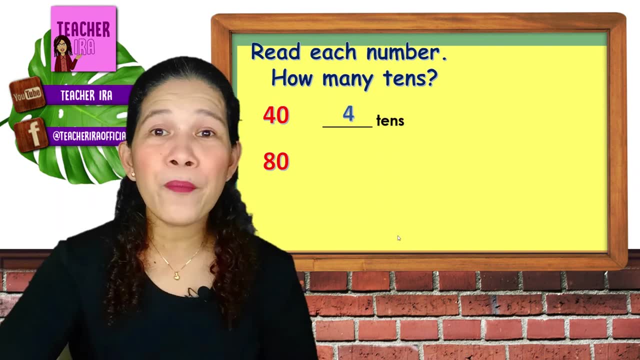 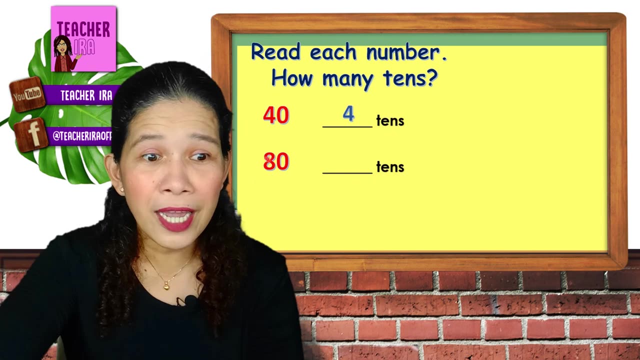 You had 40, meaning there are 4 tens and 0 ones. There are no ones. How about this number? Can you read? Yes, This is number 18.. Now, how many tens are there in number 18?? Just look at this line or this place. 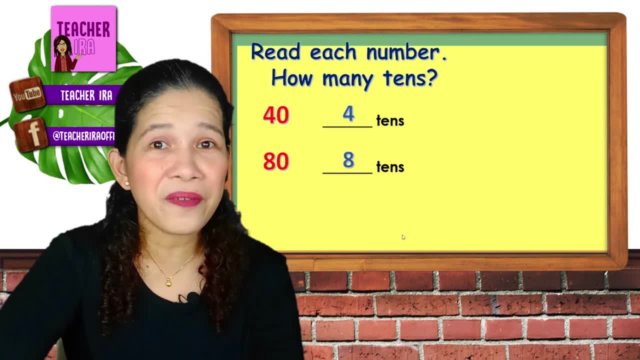 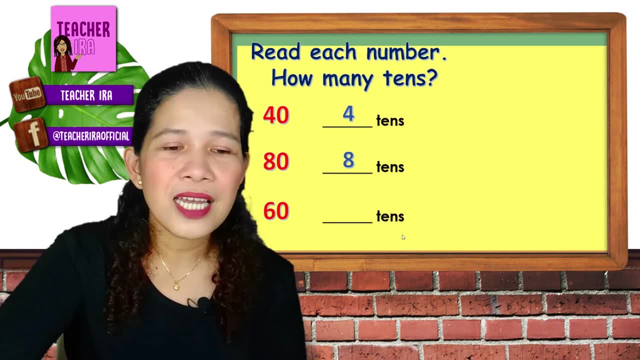 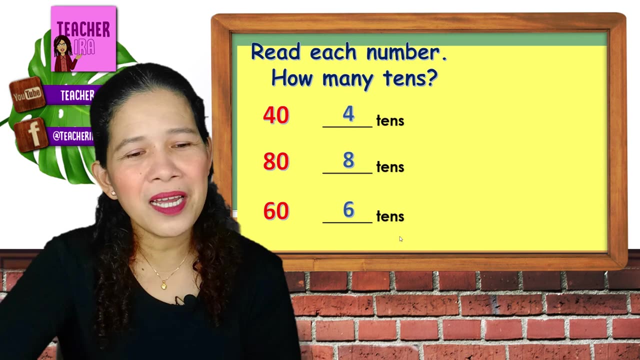 How many? Yes, So you are correct, That's 8 tens. How about the next number? How do you read this number Correct? This is number 60.. Now, how many tens are there in 60?? You are really smart children. 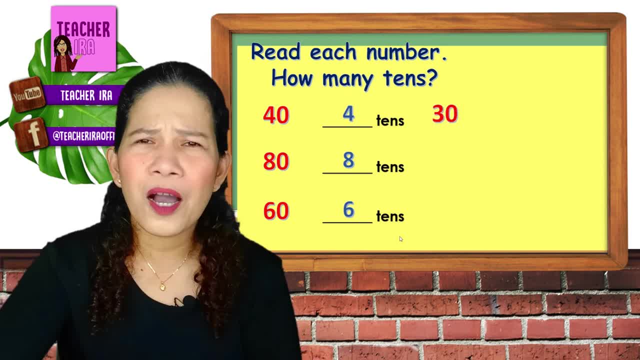 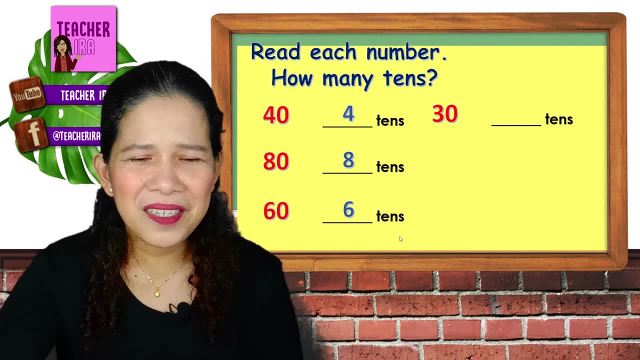 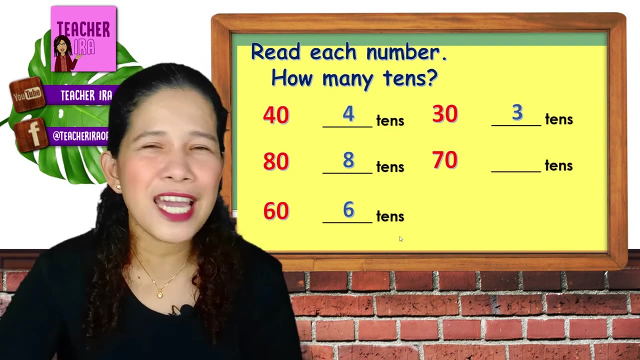 That's 6 tens. 60 got 6 tens. How about this number? Yes, Number 30.. How many tens are there? Correct, You got 3 tens there. How about this number? Yes, 70.. How many tens are there?